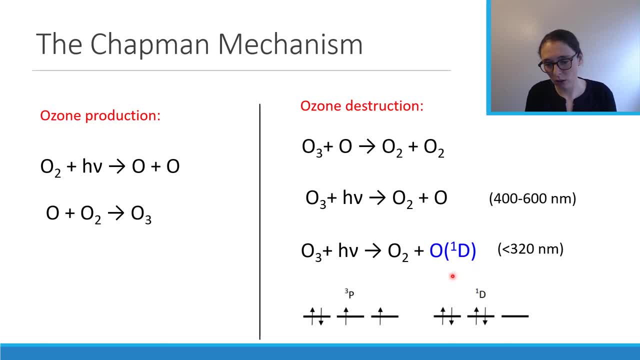 a O2 and singlet oxygen. So just a reminder from, probably, gen chem. normally this oxygen would be in a triplet state. So this is actually pretty interesting for atmospheric chemistry because the singlet oxygen is much more reactive than the triplet, so it undergoes some pretty interesting chemistry. We're not going to. 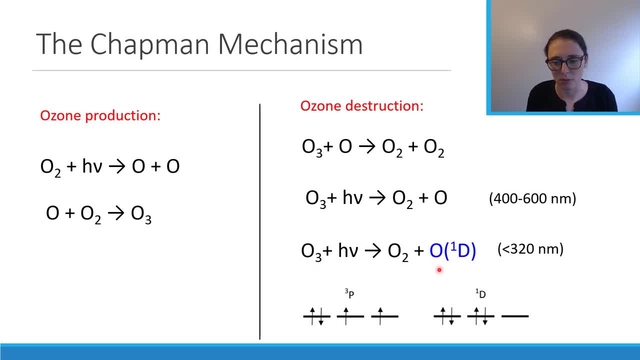 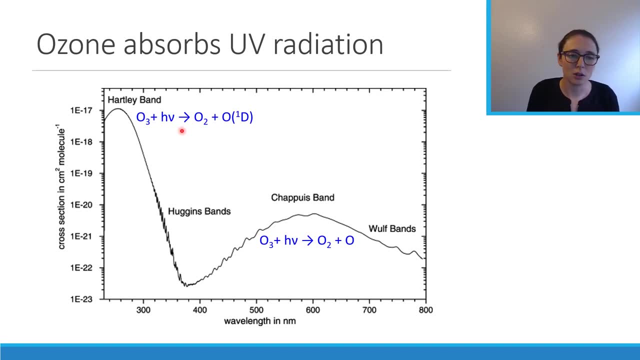 talk about that today, but I just wanted to bring that up because I think it's interesting. So ozone- we just talked- absorbs UV radiation. So our Hartley band is going to be where the ozone is absorbing that far UV, So those smaller wavelengths- is actually going to be this reaction? 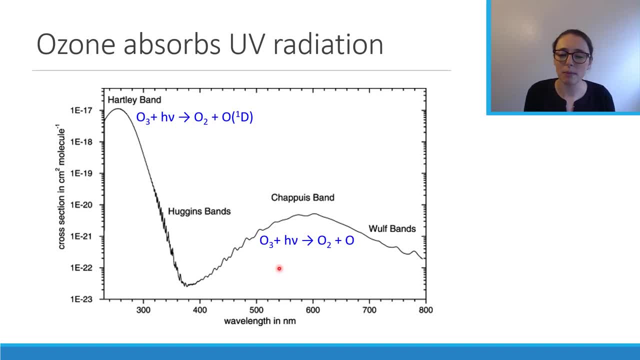 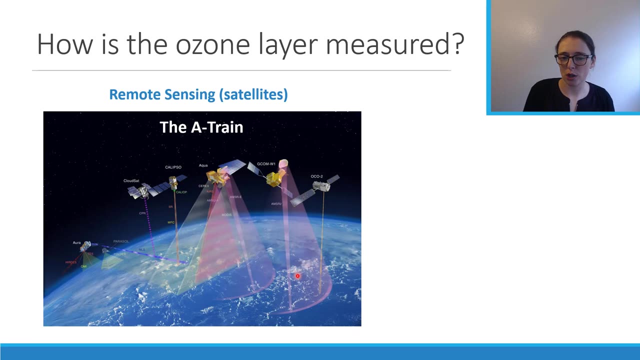 where we get the singlet oxygen, And then the Chapius band is going to be where we're just getting triplet oxygen, All right. so how do we measure the ozone layer? There is basically two major ways. The first is gonna be through remote sensing or satellites. So there's lots and lots of satellites that 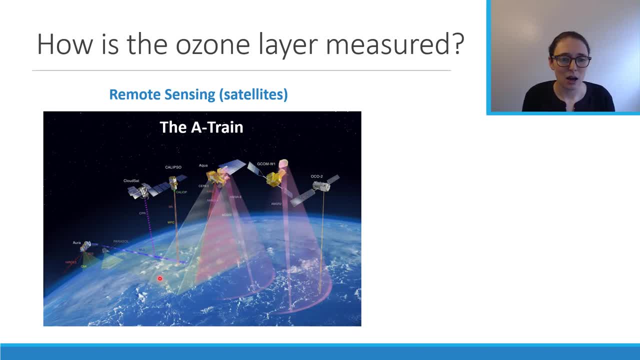 are just running around via the planet. This is just an example. This is NASA's A-train, So the ORA satellite is equipped with the ozone monitoring instrument. There's also another one called TOMS, that gets used a lot, So these essentially just rotate around the planet. 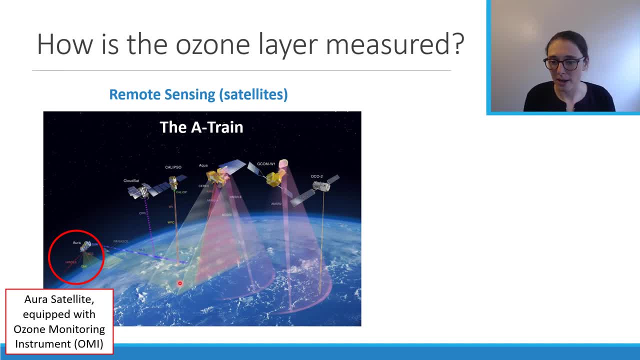 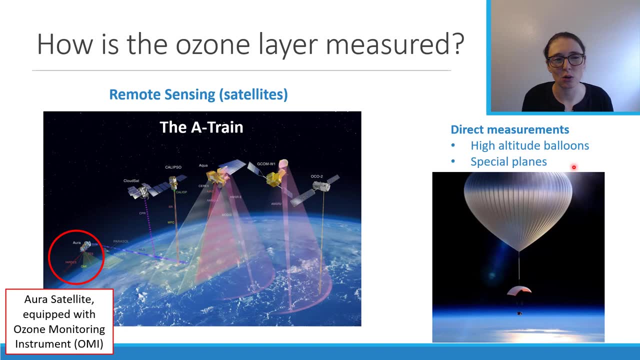 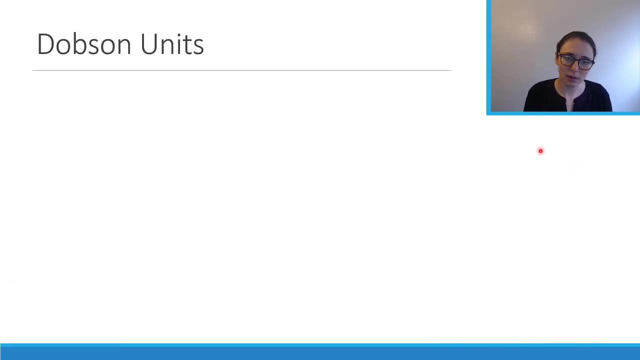 the earth, measuring the ozone layer by satellite. You can also measure ozone directly using high-altitude balloons or weather balloons. There's also special planes that can fly in the stratosphere. so we actually have done some direct measurements of ozone in the stratosphere. So when we talk about ozone, 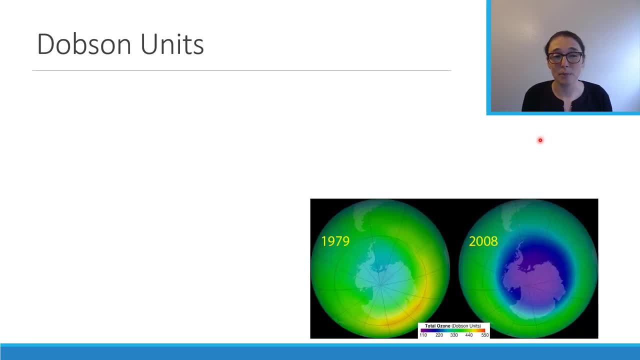 it's basically always going to be reported in Dobson units. So this is a figure showing the ozone hole and you can see here this color scale is in Dobson units. So if you're like me, before I took this class, you might be thinking. 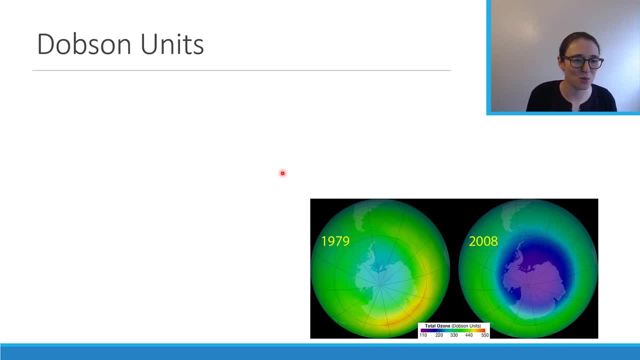 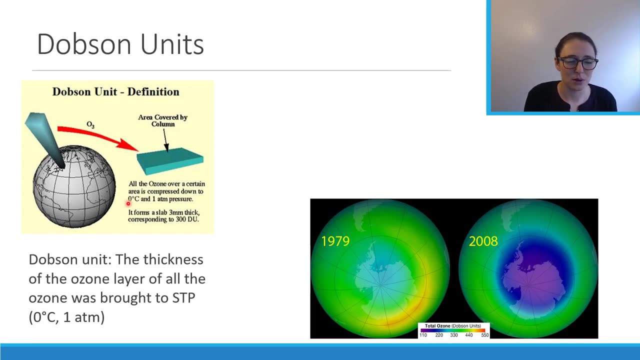 what the heck is a Dobson unit? It's actually a pretty weird unit. So basically what it says, what the unit is defined as is, if you took all of the ozone in the air column, So all of the ozone that is in the atmosphere in a 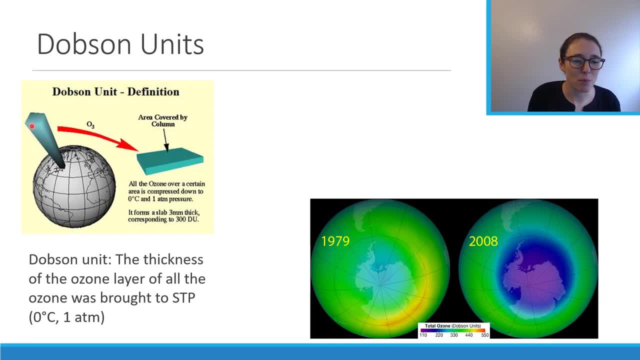 certain area And you can press. Press this down to standard temperature pressure, so 0 degrees Celsius in one atmosphere pressure. It's the thickness of all of that ozone. The global average ozone is 300 dobson units, which is 3 millimeters. 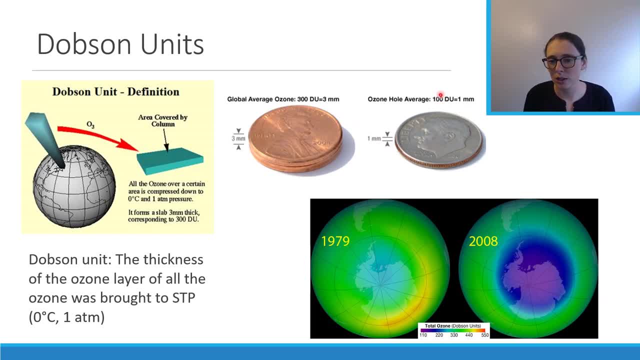 For reference, the ozone hole is only 100 dobson units thick, so that would be 1 millimeter of ozone if you took it all down and compressed it to STP. So it's kind of a weird unit. but that's what we're talking about and it's basically going. 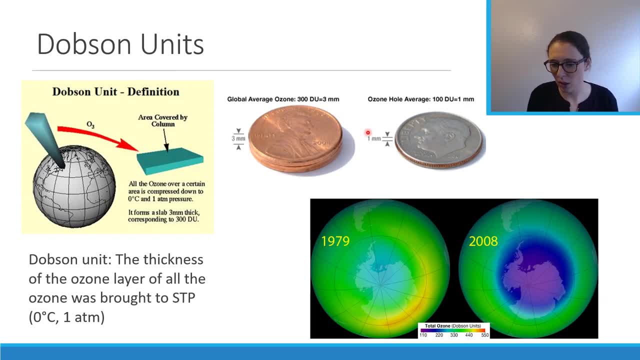 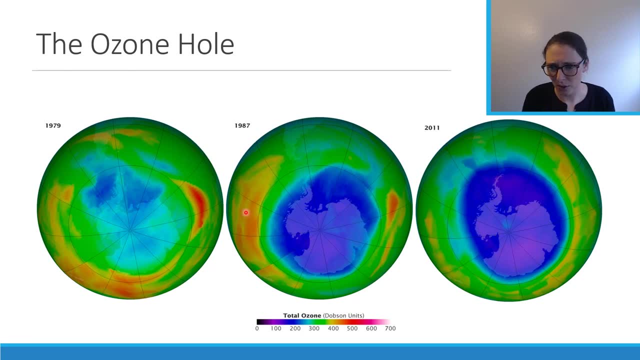 to be directly proportional to the amount of ozone in the column. So that is what we mean when we say a dobson unit. All right, so this is our ozone hole. You can see that it got worse. basically, People first started kind of to notice it in the 70s and then by 1986. 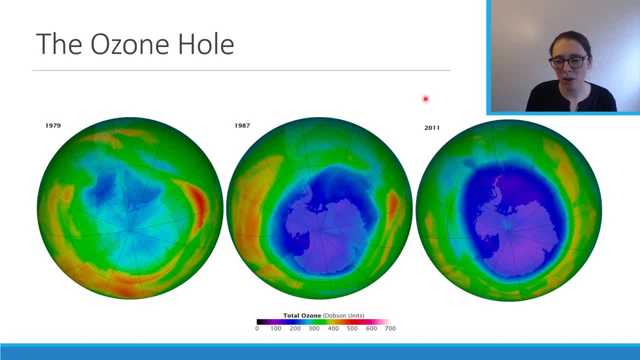 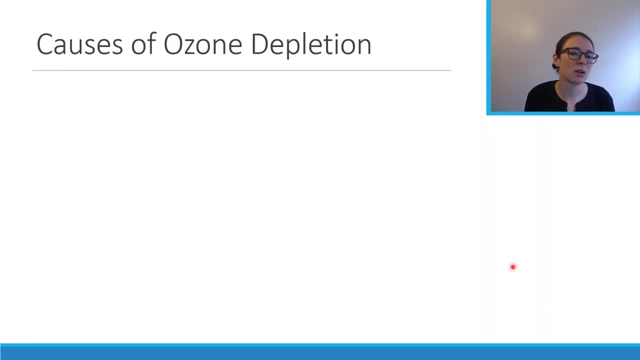 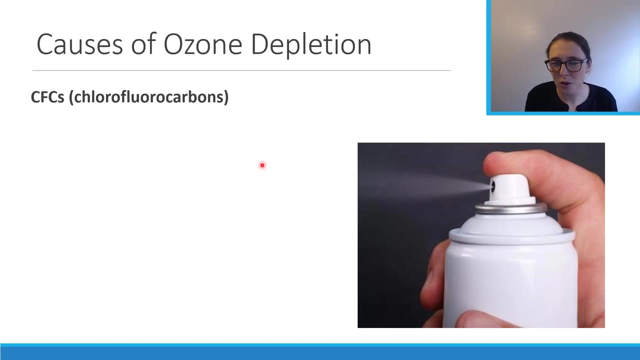 It was much more severe and then things have kind of stabilized, but still not getting much better. So let's talk about the causes of this ozone hole. So the major cause of ozone deflation is going to be CFCs or chlorofluorocarbons. 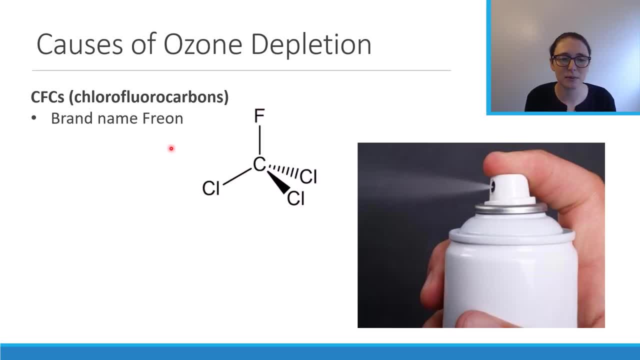 Most of you probably already knew this. The brand name for CFCs is Freon. There's different chemical variations, but basically it's just going to be a carbon backbone with a bunch of halogens or fluorine and chlorine. Fluorine and chlorine is bonded to it. 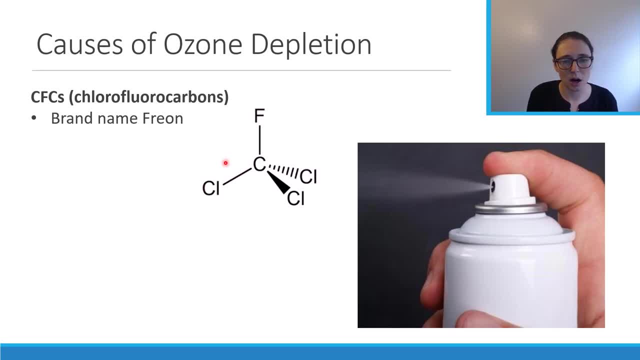 Sometimes it's a methane, Sometimes it can be like there can be two or three carbons, but this is the basic kind of structure. It's just variations on this theme. They're used as refrigerants, propellants in our aerosol cans and also as solvents. 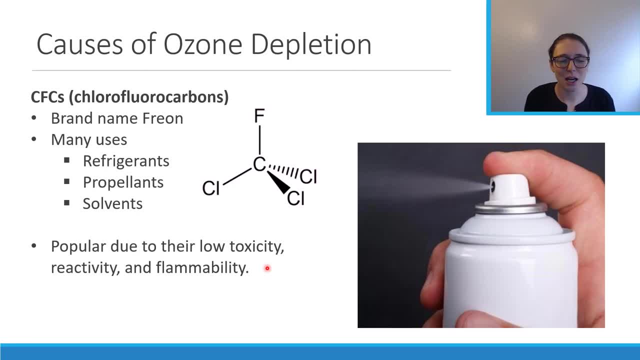 And they were really popular because they're basically non-toxic: They don't react with basically anything, They're very inert and they're not flammable. So they're really good for things like air conditioning or your refrigerator that are going to be in your house, because they can't just catch on fire and burn your house down. 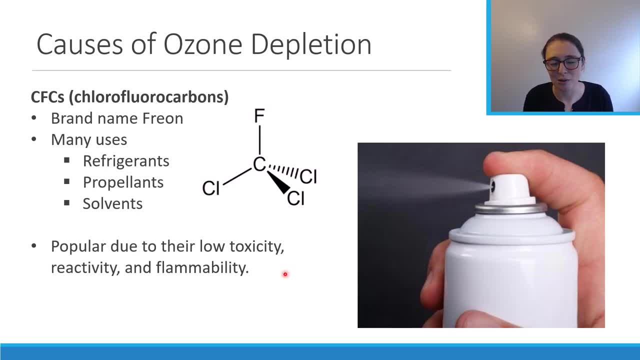 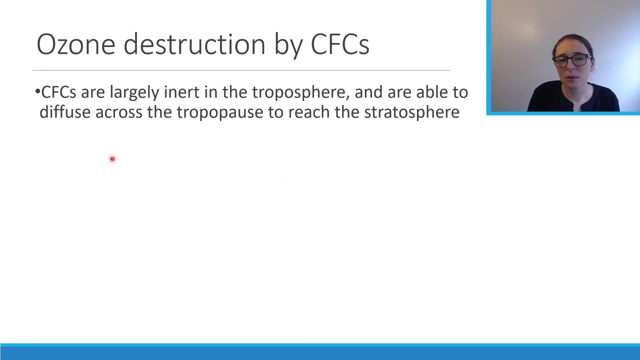 So because of all these reasons, they were really, really popular compounds. but actually this inertness, this low reactivity is one of the reasons why they were so bad for the atmosphere. So CFCs, as we said, are largely inert and so in the troposphere they don't break down. 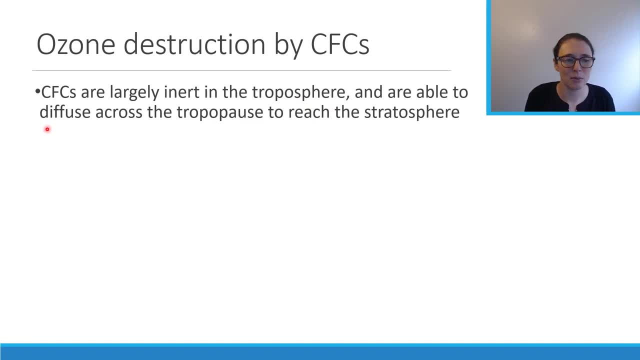 and they have really really long lifetimes, So they're basically able to diffuse across the tropopause. I realize I didn't write this down, but the lifetime of most CFCs is over 100 years. So if we remember from module two the time it takes for something to cross the tropopause. 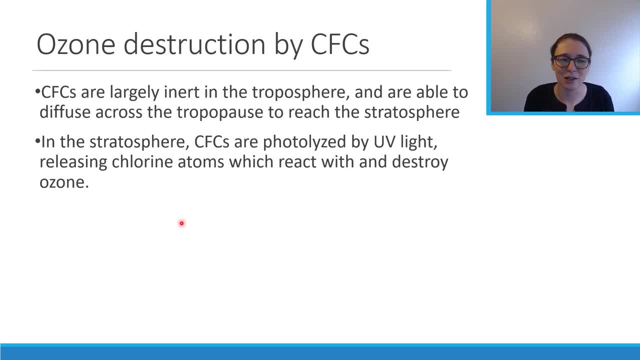 is about 5 to 10 years. That's a long time. So if the lifetime is 100 years for a given CFC, that's plenty of time for it to reach the stratosphere. Then, once we're in the stratosphere, these CFCs get photolyzed by UV light and release. 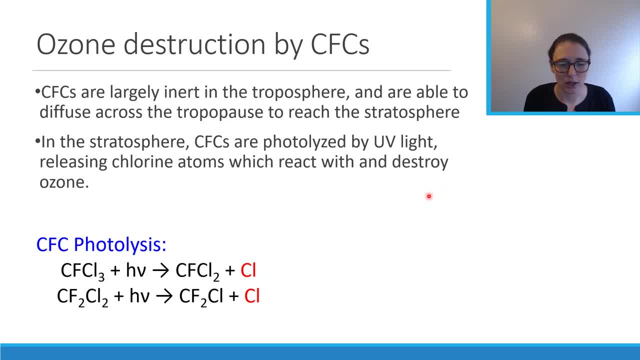 chlorine atoms and these react with and destroy ozone. So these are the reactions for CFC photolysis. I'm pretty sure these are free on 11 and 12.. I just chose two random ones. but basically these compounds plus UV light results in a 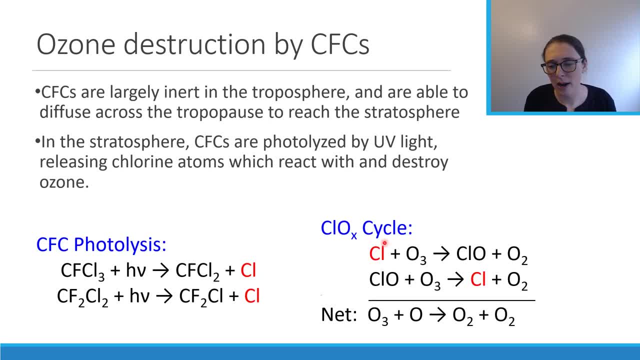 chlorine atom. So this free chlorine atom goes on to react with ozone, forming ClO, and then it actually can get regenerated. So it's not destroyed in this reaction, It just keeps reacting with ozone and the net reaction is actually just going to be. 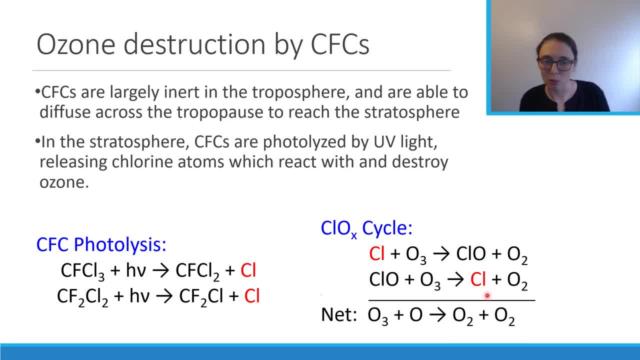 ozone going to 2O2 with this chlorine freed back up to keep reacting. So if this was able to go on indefinitely, wouldn't this happen? No, This would just destroy the entire ozone layer right. There wouldn't be an ozone layer left if this is just free to keep going. 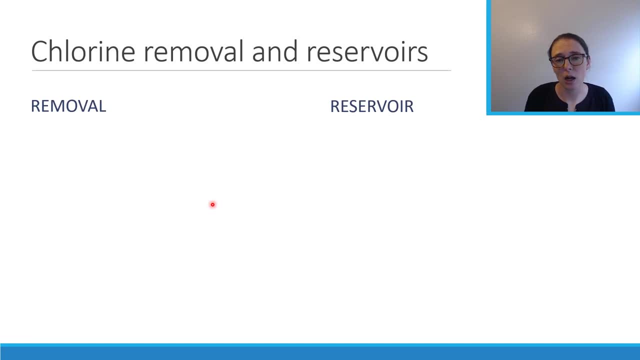 Fortunately there are ways which the chlorine gets removed and taken out of the stratosphere. So the major pathway for chlorine removal is through conversion to hydrochloric acid, So one way this could happen. we have trace amounts of methane in the stratosphere. 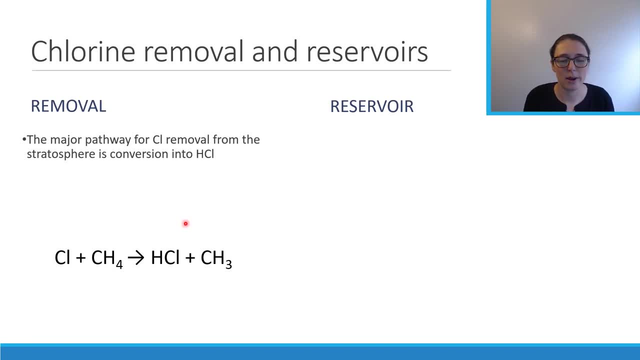 So one way this happens is chlorine reacts with CH4 to form HCl, Um And a CH3 radical, And so then a fraction of this HCl is going to make it back into the troposphere, and it will be removed from the atmosphere, essentially probably by wet deposition or chemical reactions. 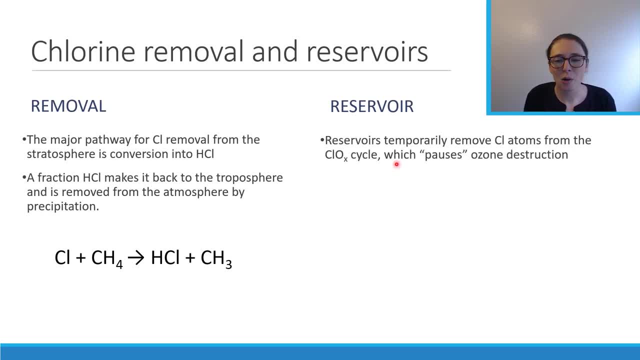 So this is one way we get rid of our chlorine. Another way we can get rid of the chlorine is basically to put it into a reservoir species. So these reservoirs are going to temporarily remove chlorine atoms From the ClOx cycle. So they're not being permanently removed and taken away, but it essentially pauses the 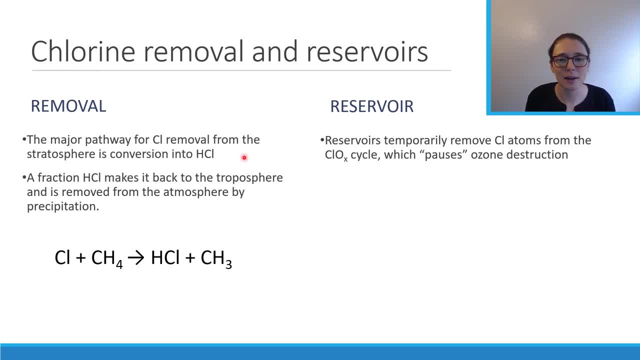 ozone dissection, So we can think of our removal as like a stop button And this is our pause. So the primary way this happens is through a reaction with NO2.. And so through this reaction we get ClONO2.. And then the reverse reaction of this: it can decompose in the presence of light. 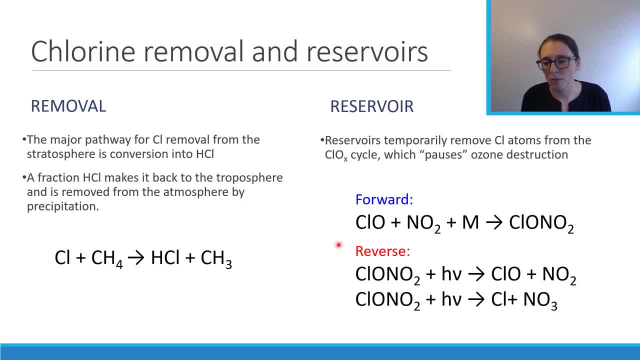 So it will go from ClONO2 back to ClO or a chlorine atom, depending on the wavelength of the light. So depending on you know the rates at which these are happening, this can actually take a fair amount of chlorine out of the ozone destruction cycle. 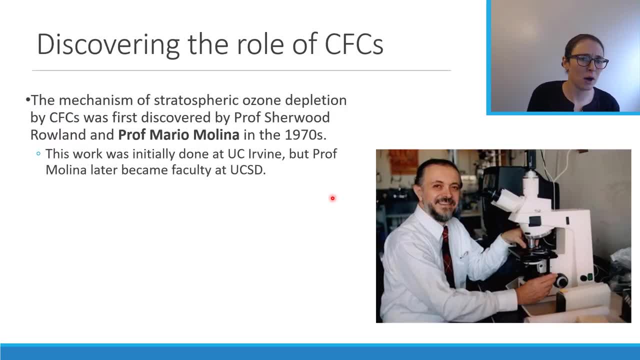 All right. so before I move on, I just briefly wanted to talk about discovering the role of CFCs in stratospheric ozone depletion. So this was actually first discovered by Professor Sherwood Rowland and Professor Mario Molina in the 1970s. 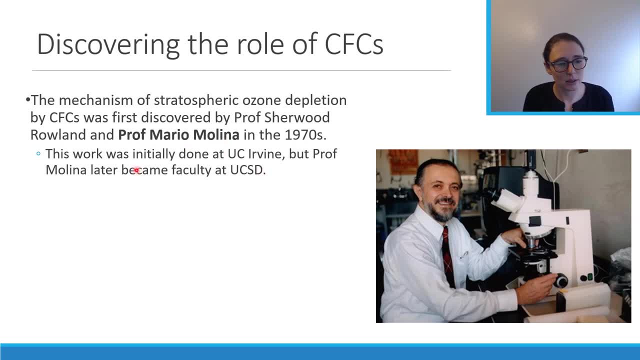 If that name, Mario Molina, sounds familiar to you, it's actually because Professor Molina is a member of the chemistry faculty here at UCSD. This initial work in the 70s was all done at UC Irvine, but then Professor Molina went. 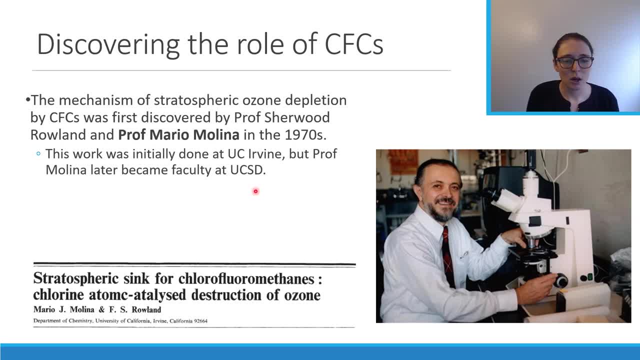 on to become a faculty member at UCSD. This is their first paper on this, So this is for 1970.. 1974, so. stratosphere sink of chlorofluoromethanes, chlorine atom, catalyzed destruction of ozone. 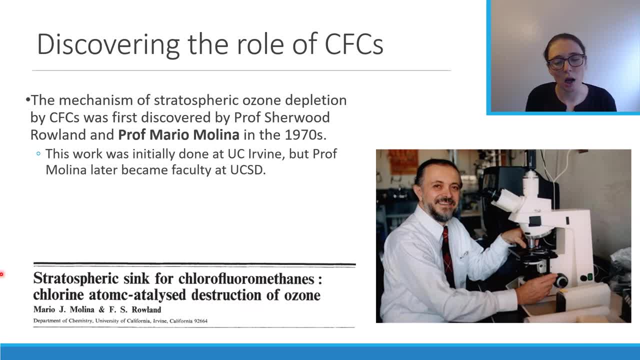 So this paper was a huge deal and it really got the ball rolling on the impacts of these CFCs on ozone depletion and they continue to do a lot more work that elucidated the full chemical mechanisms that these compounds go through And in 1995.. 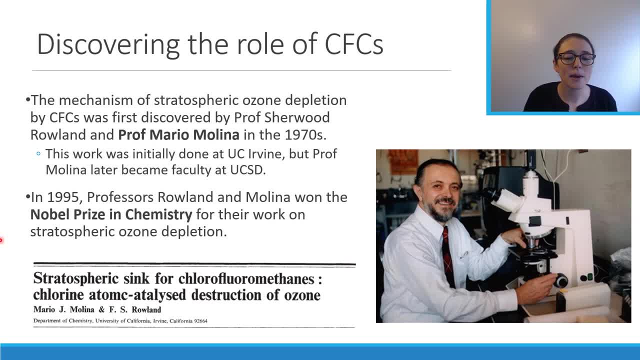 Professor Rowland and Professor Molina won the Nobel Prize in Chemistry for their work. They shared this prize with Paul Crutzen, who is someone who is a scientist who discovered the depletion of ozone in the stratosphere, So this was a huge deal. 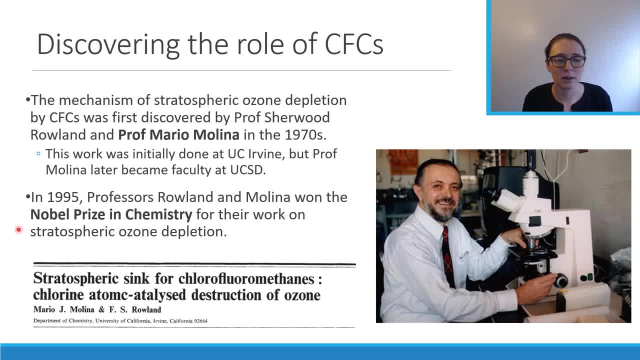 To date, this is the only atmospheric chemistry or only Nobel Prize that has gone to atmospheric chemistry. So this was a huge deal. Professor Molina normally lectures for this class, but given all the craziness and the move to online classes, Unfortunately he's not available to lecture for us this year. 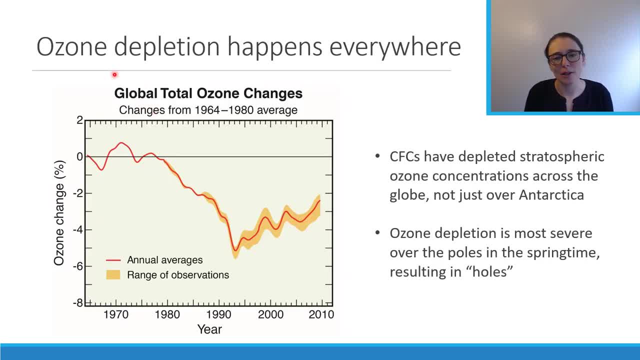 All right. So ozone depletion happens everywhere. We really concentrate on the Antarctic ozone hole because it's the most severe occurrence of ozone depletion, But actually, globally averaged, the total amount of ozone in the stratosphere has gone down in the mid 90s. 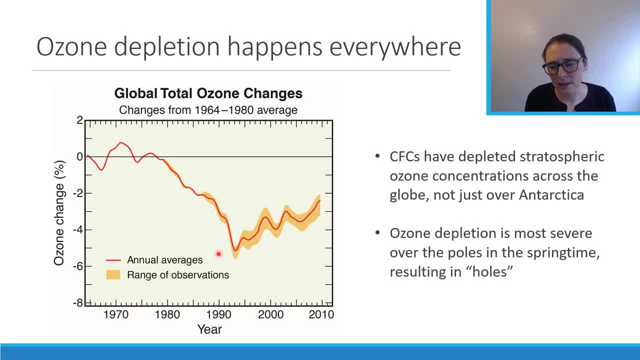 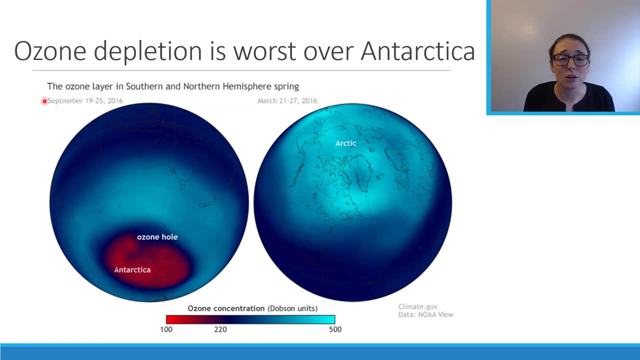 It reached a low of about 5% below normal. It's slowly recovering, So it's not a huge change. but ozone depletion actually was a global problem. It wasn't just a problem that was happening over Antarctica. So, as we just said, ozone depletion is worst over Antarctica. 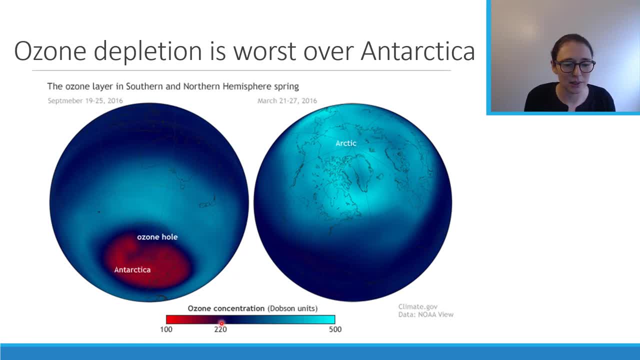 So that's where we get this really severe hole, where the ozone is like half or a third of what it's supposed to be. We also get an Arctic ozone hole some years or at least more ozone depletion over the Arctic, But it will not be as severe as over Antarctica. 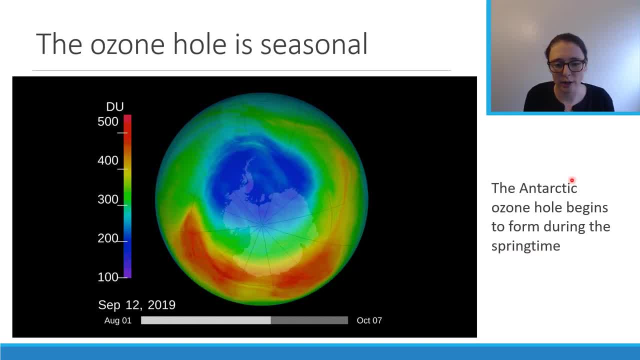 The ozone hole is also seasonal, So it begins to form during springtime. So this is the Antarctic ozone hole, So southern hemisphere spring is going to start around August, so our fall basically. So during the springtime the ozone hole will start to form and get more and more severe. 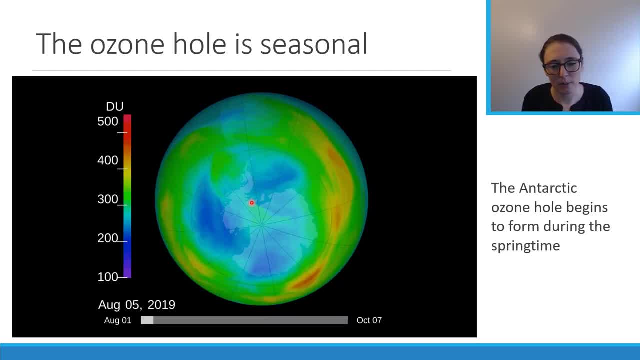 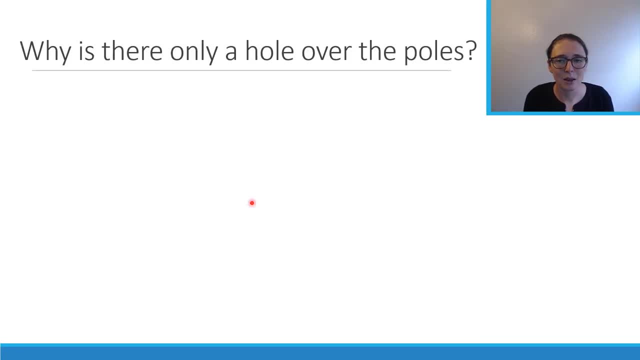 So you might- some of you guys probably have learned about this already, but others you might be wondering: Why does this happen? Why is this only forming over Antarctica in the springtime? And the answer is: clouds. So while in general our stratosphere is really dry and cloudless during the winter, in the 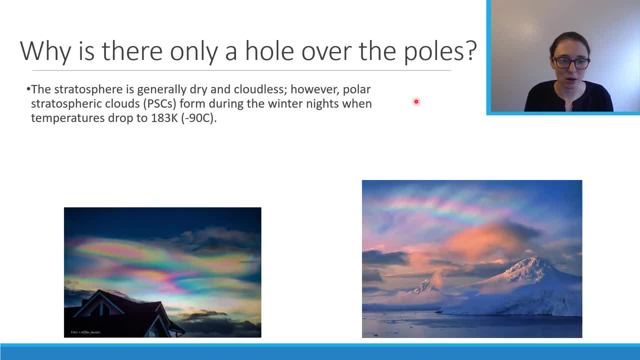 poles, we get the formation of polar stratospheric clouds. So these clouds are forming when the temperatures drop really, really cold. They're made of ice, So regular water ice, Which provides a surface for reactions to happen on, But they also contain frozen nitric acid. 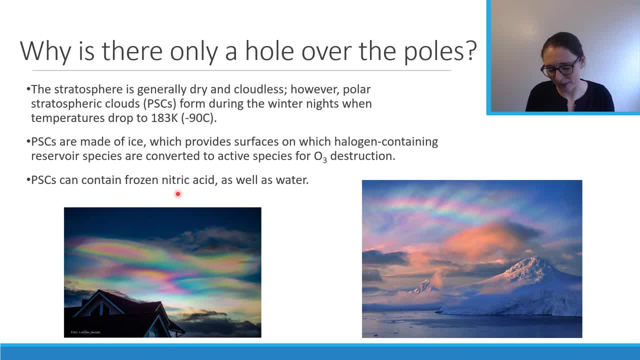 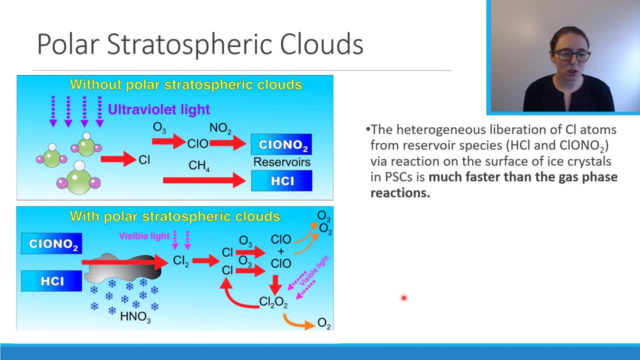 So they're not just pure water, they're actually frozen nitric acid droplets. Okay, so the basic way that this works is that our reservoir species are going to react on the surface of these ice crystals, and the reaction to free up these chlorine atoms is: 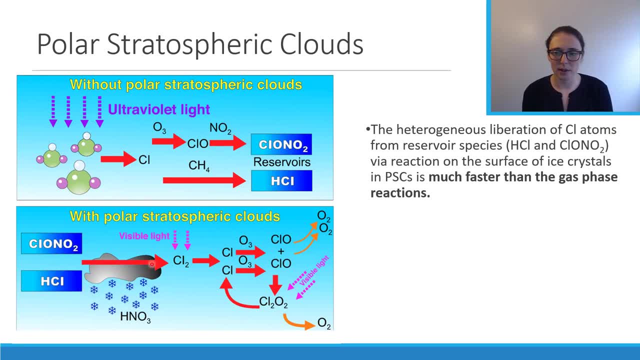 going to be much, much faster When it happens on the surface of the ice crystals than it happens in the gas phase. The other thing that happens is so we have our two reservoir species, HCl and ClNO2, reacting with one another on the surface of the ice crystal. 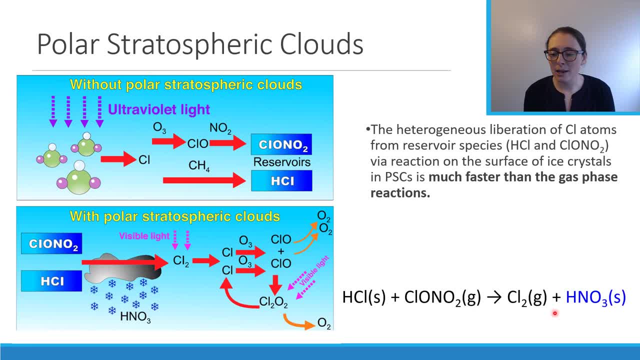 It forms chlorine gas, and then this nitric acid gets left tied up in the ice crystal as frozen nitric acid. So this NO2, or HNO3, is nullified. Okay, Okay, Okay, Okay, Okay, Okay Okay. 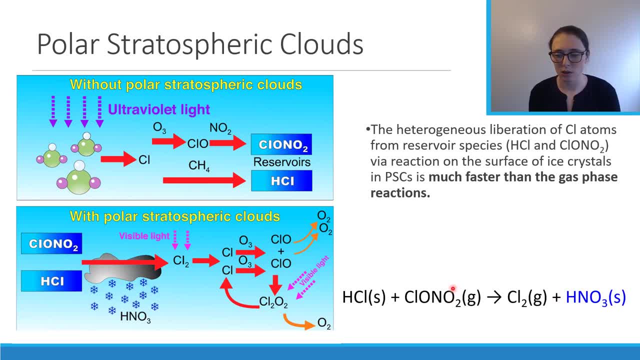 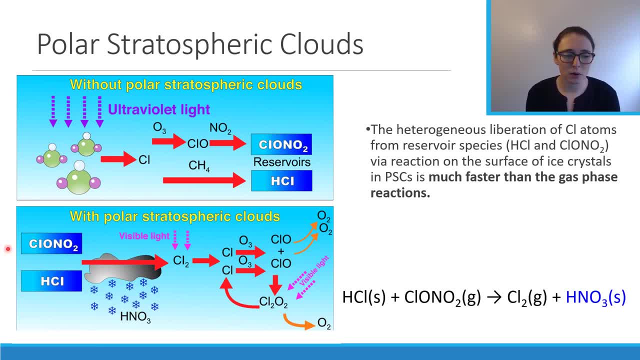 So essentially what happens is the polar stratospheric clouds enable all of the reservoir species to be destroyed and they can't be reformed, and then all of this chlorine gas builds up in the stratosphere, And so these clouds are forming over the winter, and it's dark, there's not a lot of light. 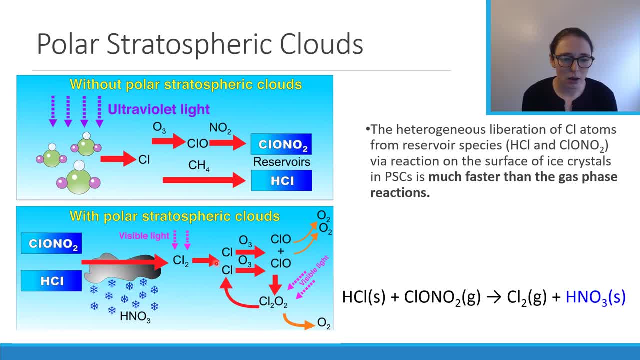 in the poles in the winter it's almost total darkness. So all of this chlorine builds up, and it builds up and it builds up all winter. then when we hit spring we get a bunch of light and this chlorine decomposes into chlorine atoms in the presence of UV light and causes a huge catalytic. 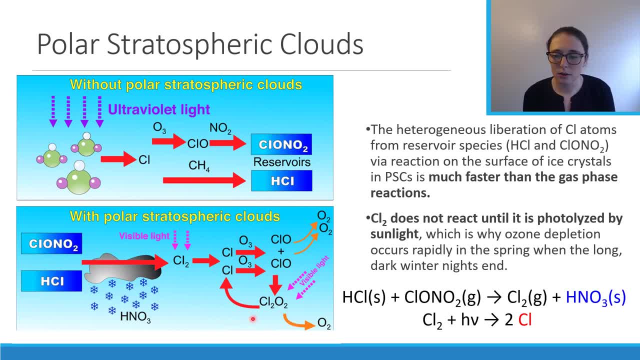 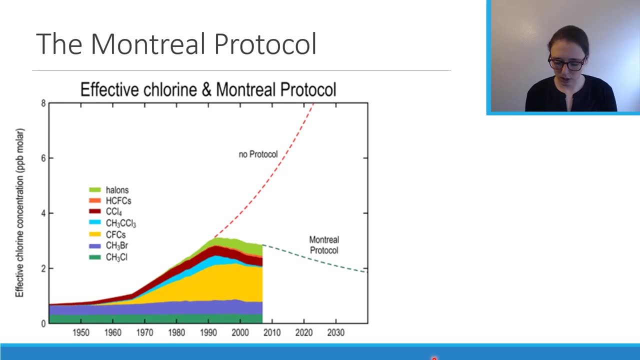 destruction of ozone. So this is essentially why we see this huge depletion of ozone in the polar regions in the springtime. Alright, so let's talk about the Montreal Protocol. So the Montreal Protocol was an international treaty designed to phase out substances which deplete the ozone layer. So 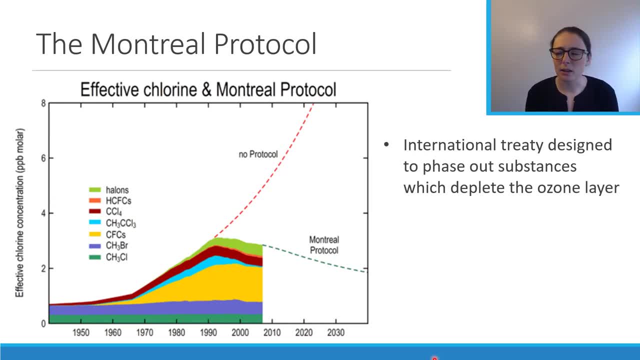 basically by the mid 80s, there was a pretty big scientific consensus that we needed to stop emitting CFCs and phase them out. There was also a lot of cooperation from the companies- chemical companies that were manufacturing CFCs- to develop alternative compounds. So this would be our H-CFCs. 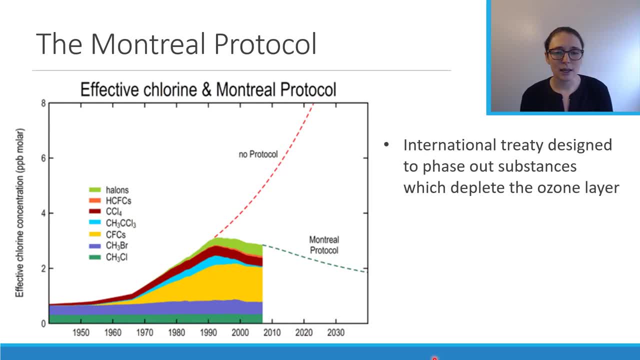 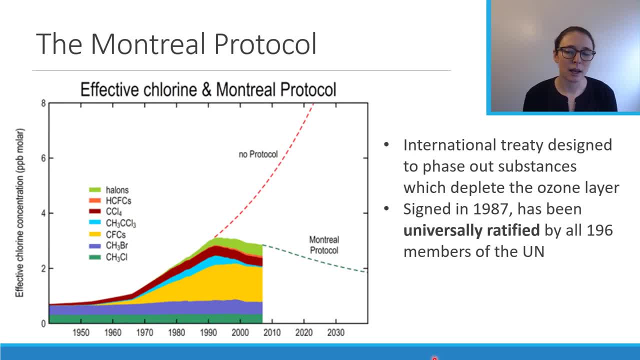 treaty to phase out CFCs. It was signed in 1987 and it was universally ratified by all measure members of the United Nations, which is pretty outstanding, And it set a timetable for phasing out HFCs and then H-CFCs, as 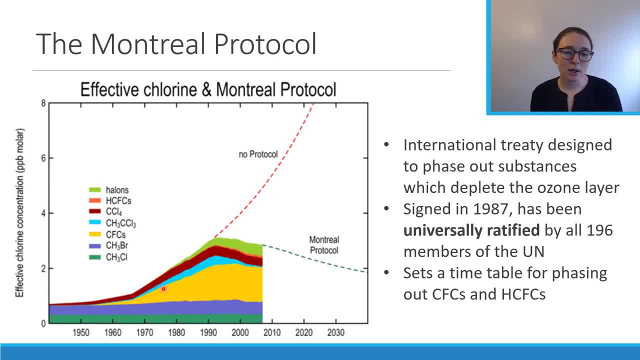 well. So we can see it's been quite effective in reducing the amount of chlorinated substances in our atmosphere. Without the protocol, we were basically in an exponential increase of all of these chlorinated compounds. With the Montreal Protocol, we are slowly phasing these things out. There are definitely 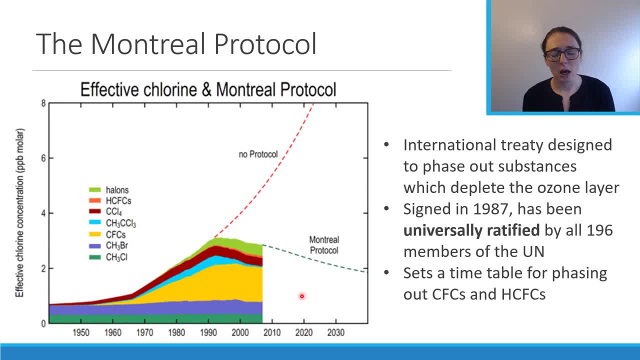 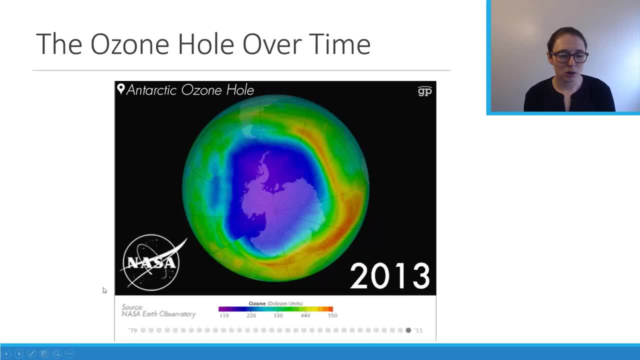 scientists who think that it's not moving fast enough, but it's definitely a huge improvement from this exponential growth trend that we were on. So this is a video that I'm going to show you. This is an investigation clip from a video showing the ozone hole over. 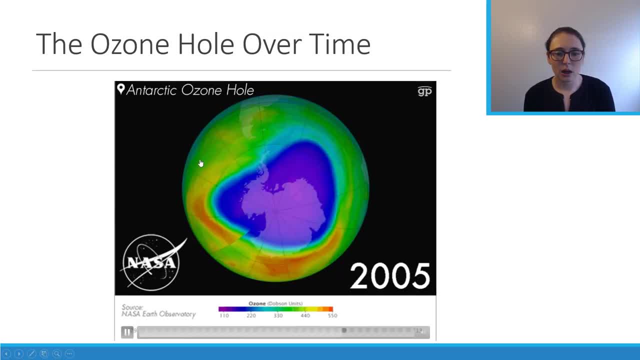 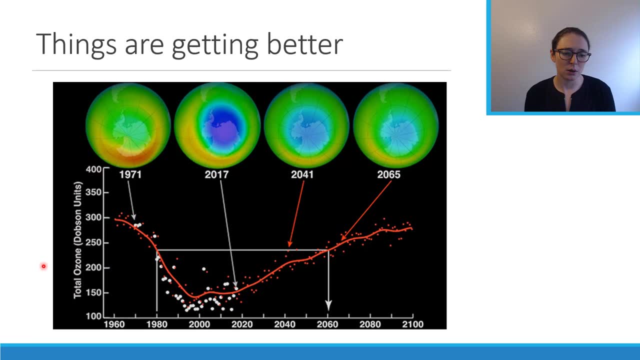 time. So we can see that throughout the 80's it got worse and now it has kind of plateaued. So when we look at this plotted- just the total ozone over Antarctica- over time we can see that the problem got a lot worse Throughout the 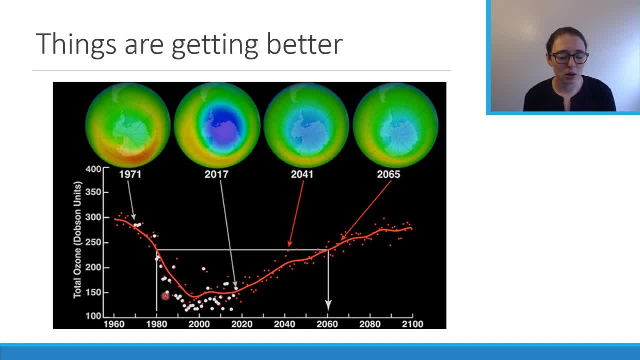 70s. we reached basically our worst ozone hole in the 90s or so, and then slowly, with the implementation of the Montreal Protocol, we have basically drama. That's one good thing, though, So we can see that through that. we can see that through the entire world. So actually since the 1980s, where we now are realizing we were, we're thinking about the plans to open data centers like that and particularly do a deeper research, that we can think about control of their building systems, because they're It's so important that it creates problems. so I don'tand that we as individuals don't. 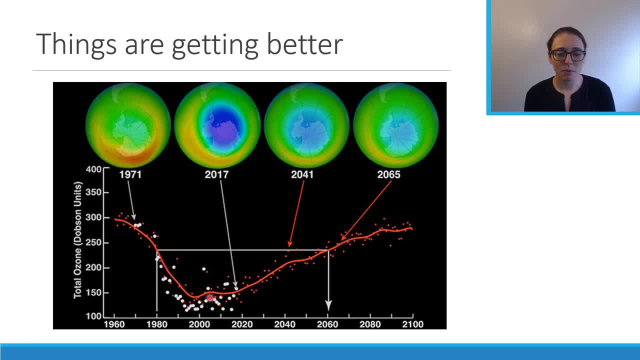 things are getting better. however, we're not projected to see a full recovery of the ozone hole, really until past almost 2100. it's gonna take over 100 years to recover from the effects of CFCs and that's because their lifetime is so long. 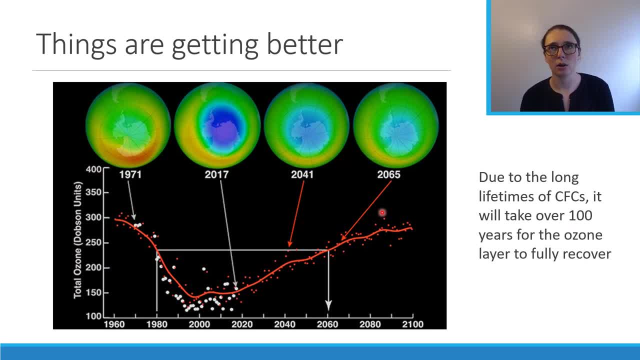 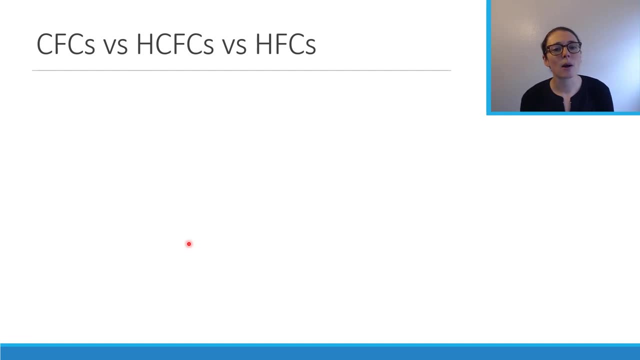 even though we have stopped emitting them, their their effects are still felt on our atmosphere because of their long, long lifetimes. but things are getting better and the Montreal Protocol is widely regarded as a major success in environmental regulations. alright, so let's talk about some of the things that 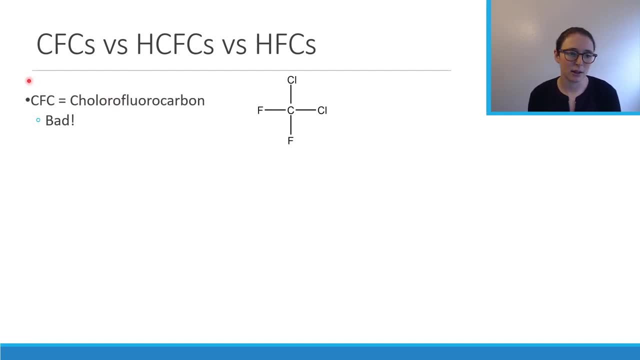 we have replaced CFCs with. so our CFCs? obviously they're bad, they cause the ozone hole. the next class of compounds that people came out with were HCFCs or hydrochlorofluorocarbons. so basically you can see here, no, 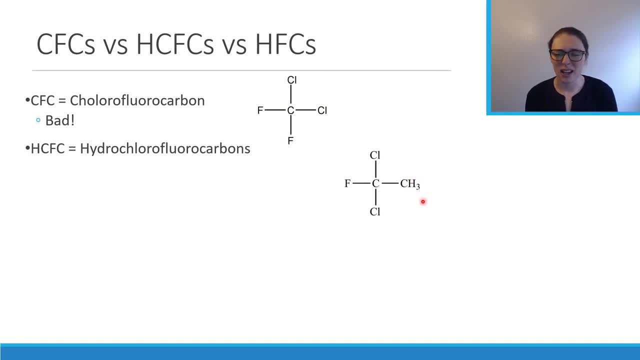 hydrogen's on these HCFCs we have hydrogen, and the reason they added these is because the CH bond will react with OH radical in the troposphere and thus shorten the atmospheric lifetime. so this is a little cartoon I made. so this is our HCFC and you can see that our little 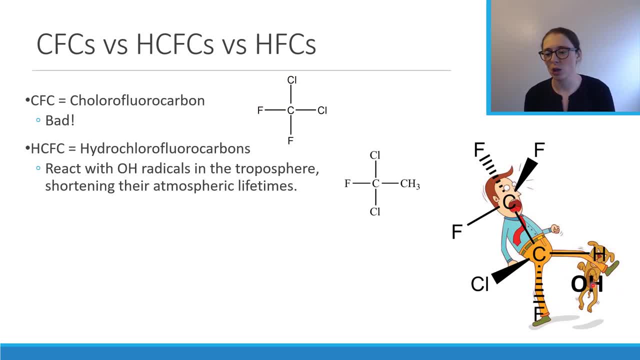 OH radical is attacking this carbon hydrogen bond. so by adding that CH bond, we've essentially given OH radical something to attack, and it can break down these compounds. the unfortunate part of these things is, though they work really well, they still contain chlorine in their lifetime is, I'm gonna say, 10 to 15 years is the. 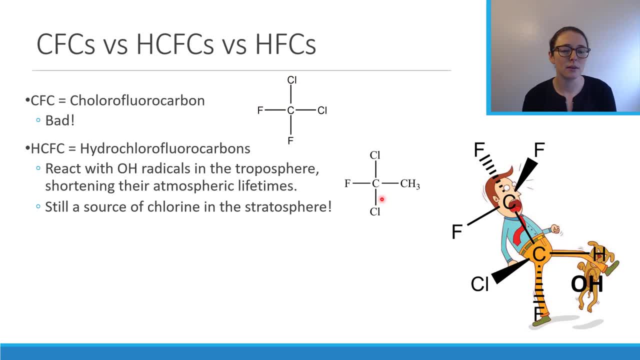 typical lifetime of HCFCs. it's a class of compounds and on individuals, so there's like a range, but they still contain chlorine and they still stick around long enough that they're able to get into the stratosphere, so that's not great. so now the next generation of compounds is HFCs- hydrofluorocarbons. 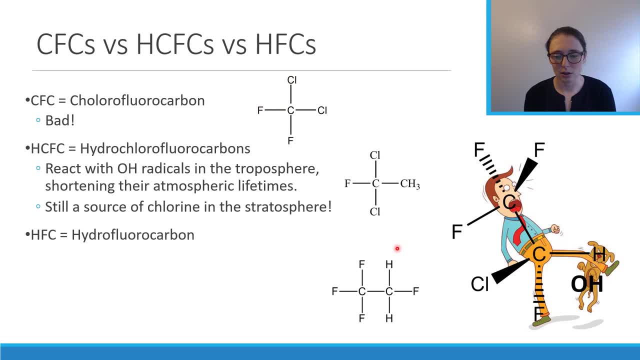 so if you notice no chlorines in sight, they still have these CH bonds that can be broken down by our OH, so these are good because they don't contain chlorine. the problem with these compounds is that they are potent greenhouse gases. so essentially we're fixing one problem- ozone depletion- but then by adding these. 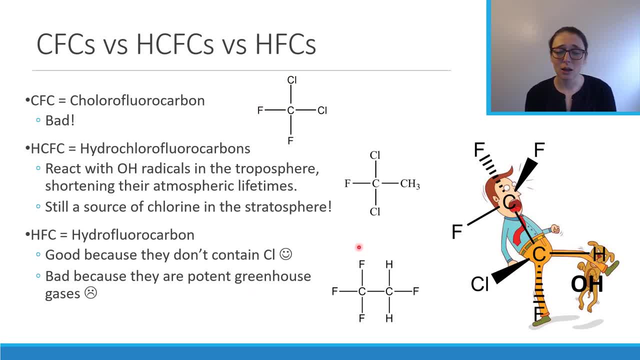 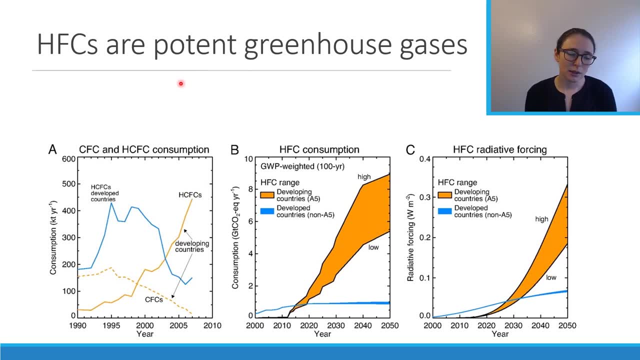 compounds to our atmosphere, we're adding greenhouse gases and although their lifetime is much shorter than that of a CFC, it's still somewhere around 10 years. so, as I just said, HFCs are potent greenhouse gases and the use of them is expected to go up as more countries industrialize and more people want. 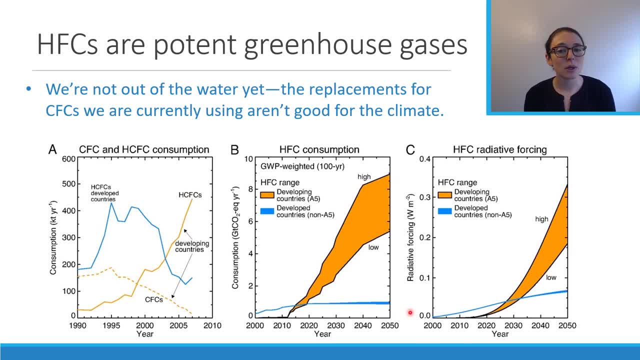 refrigerators and air conditioners and all the things that we use these compounds for. so we're really not out of the water yet, and we need to develop new alternatives for CFCs that are good for the climate and don't hurt the climate, but definitely in terms of energy and hydrogen there's a lot of different ways. 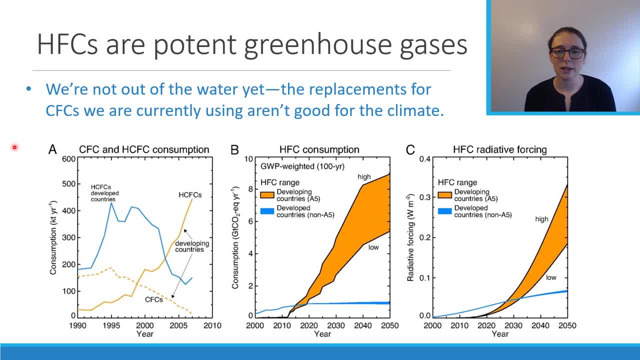 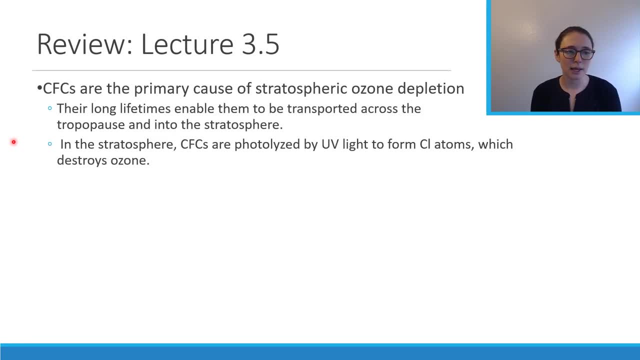 But definitely in terms of energy and hydrogen. there's a lot of different ways. terms of fixing the ozone layer, the montreal protocol has been a massive success. okay, so that is the end of lecture 3.5. just to briefly recap: um cfcs are the primary cause of stratospheric. 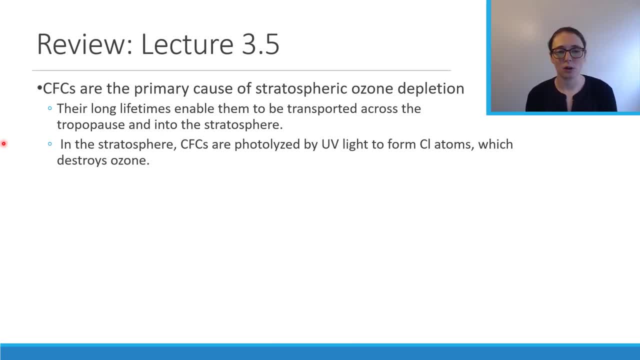 ozone depletion. their long lifetimes enable them to be transported across the tropopause and into the stratosphere. the cfcs get photolyzed from chlorine atoms, which basically destroys ozone, and we talked about how ozone depletion is most severe in polar regions in the springtime, because